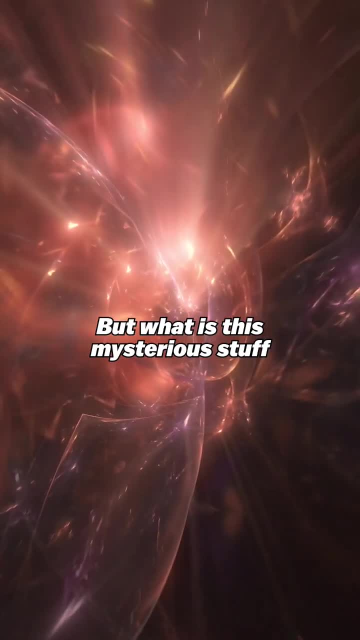 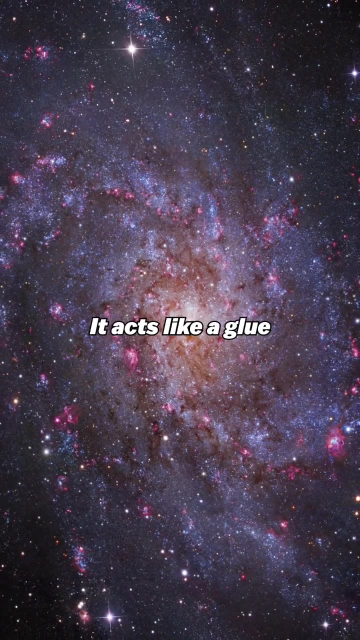 energy and dark matter. But what is this mysterious stuff that we can't see or touch? Well, dark matter kind of works like an attractive force. It acts like a glue that holds all of our galaxies together. Dark energy, on the other hand, can be thought of like a repulsive. 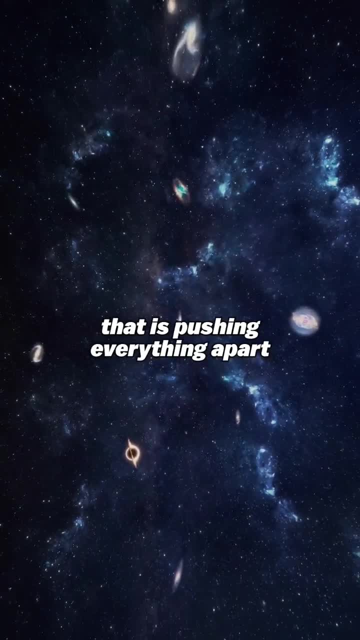 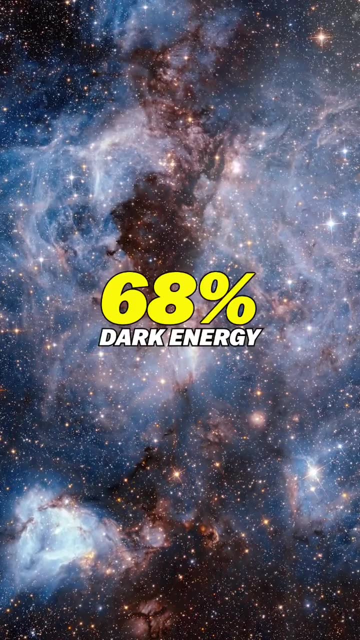 force. It is an extremely strong force that is pushing everything apart, causing the universe to expand. We think the universe is made up of around 68% dark energy and 27% dark matter. This is really one of the biggest problems in physics, So if you can solve it, I can. guarantee there is a Nobel Prize waiting for you. 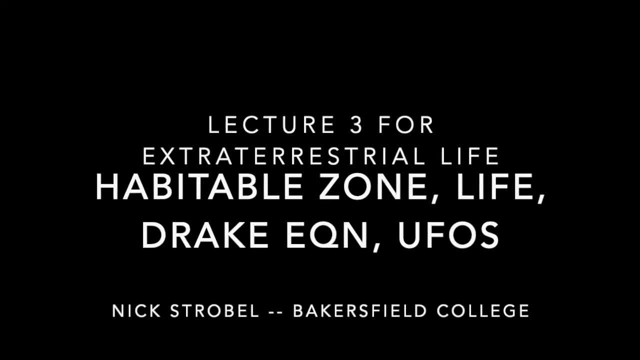 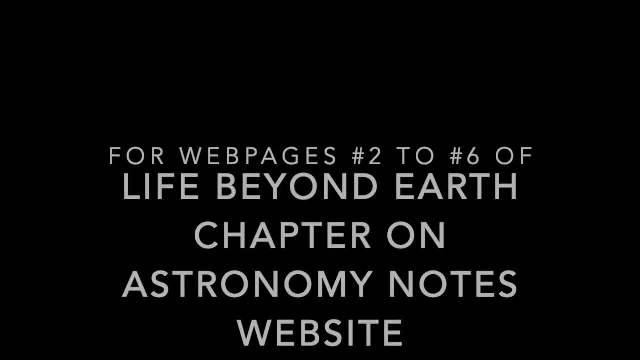 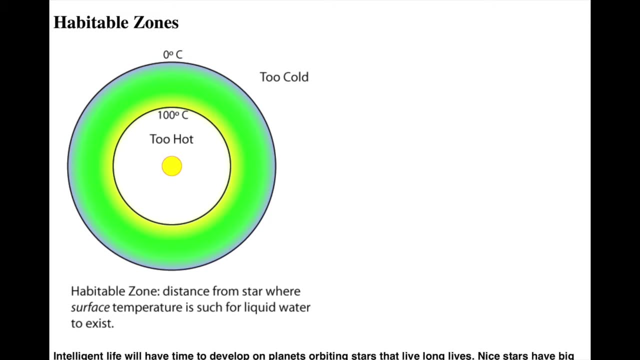 Next slide. Before I talk about biomarkers, let's look at this idea of the habitable zone. There is a range of distances within which the surface temperature could be nice enough for liquid water to exist on the surface. Note the water bias and the surface life bias- here, The type of life we're going to be able to detect. 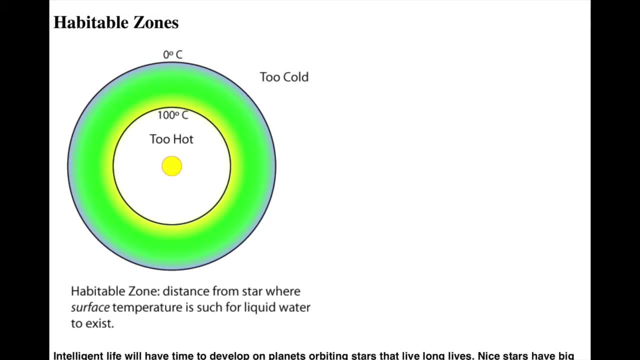 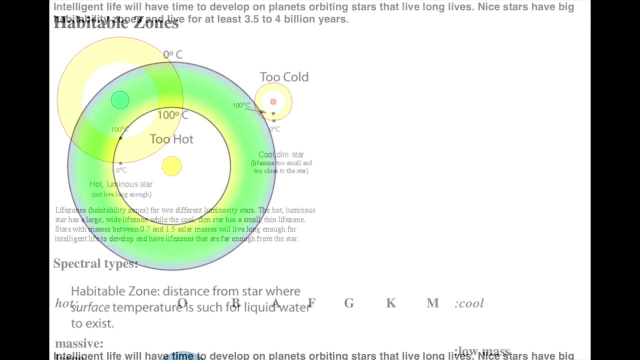 from tens to thousands of light years away is life on the surface of the planet, and even with the water limitation we're expecting to find a lot of suitable planets. The habitable zone of a hotter main sequence star will be farther out and wider because of the hotter. star's greater luminosity. Using the same line of reasoning, the habitable zone of a cooler main sequence star will be closer to the star and narrower. Unfortunately, the hot, luminous stars with big, wide habitable zones live very short lives If life on Earth is. 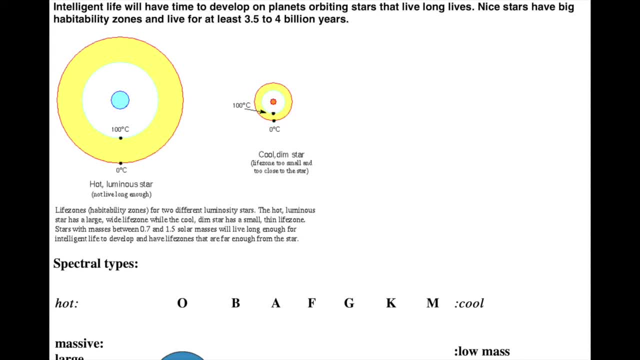 any sort of guide for how long it takes intelligence to arise, then we're going to want to focus our attention on stars that live for at least 3.5 to 4 billion years. On the other hand, stars smaller and cooler than the Sun are very common with the so-called M-dwarf stars. 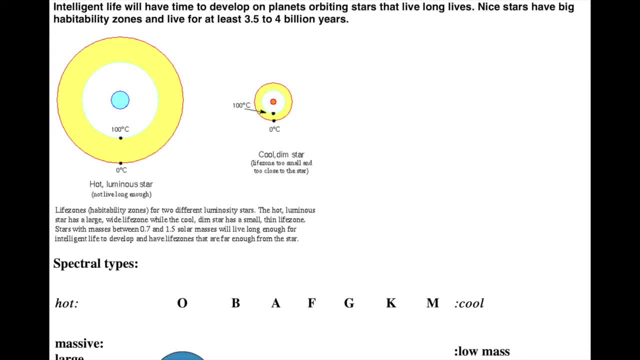 They have very small, thin habitable zones. Exoplanets in that close to their star will probably become tidally locked, like the Moon is to the Earth, so that one side always faces the star and the far side is in perpetual night. One side hot and the other side so.